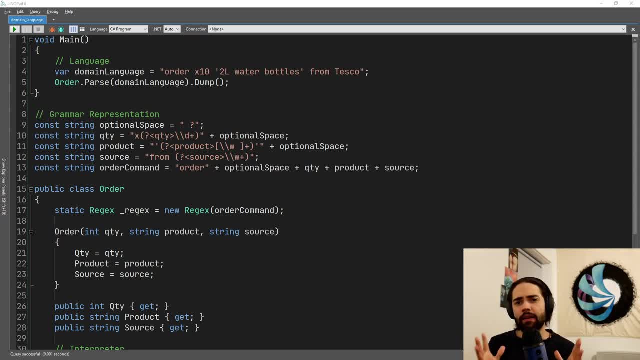 and then we're going to execute some code behind it. This pattern is very easy to recognize and understand what it should do. Its complexity lies in its implementation and, I would say, its scarcity. There's not many implementations going about Usually, if they get implemented- 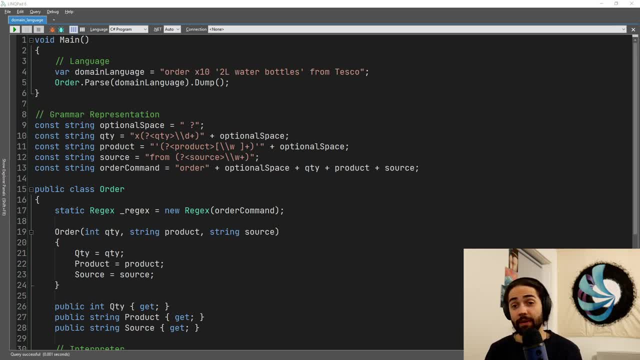 once they will get reused. We'll take a look at some examples of very successful applications of the interpreter pattern. Nevertheless, if you're enjoying these videos, don't forget to like subscribe. If you have any questions, as always, leave them in the comment section. 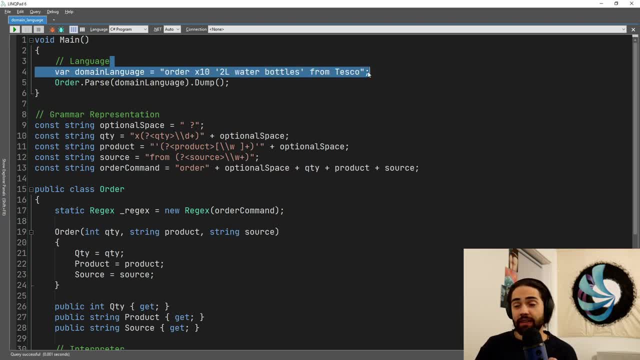 Let's dig in into the example that I have here Specifically. the language I've decided to choose is not for us programmers, although we have our own interpreters meant for our use case. This is more for the business side of things. So let's say I am in a retail business. 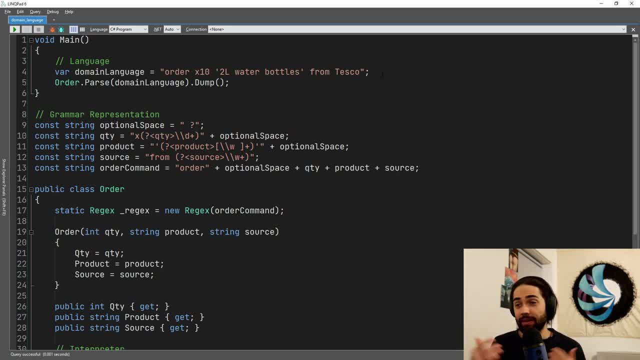 where we sell order loan. I don't know things right. Products going about back and forth And the general thing is filling out a form with products and whatnot or going to someone's website. It's too long, right. I can just say: buy me 10 bottles of Coca-Cola and one croissant. 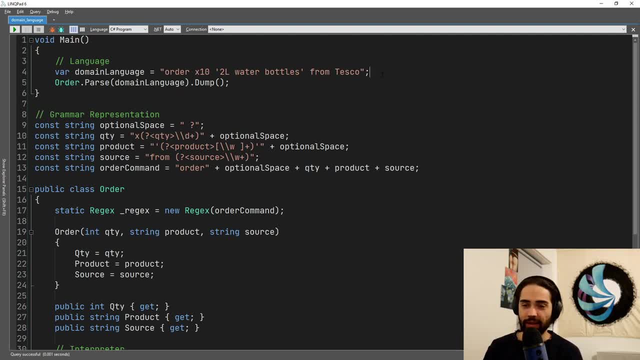 that has chocolate in it or something like that, And then the order will get filled out automatically, It will get paid by the system And that's it right. And I'm going to put that order through Alexa or Google Home or whatever. 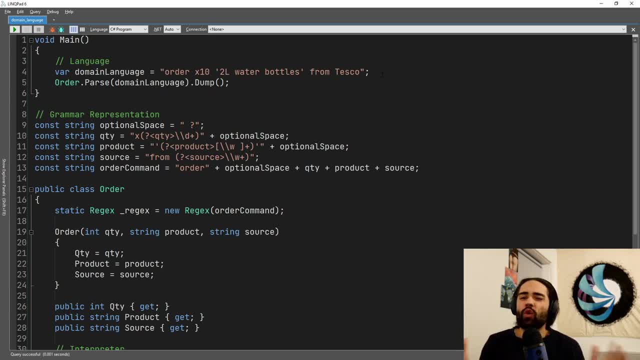 one of the voice devices or Siri. I don't want to sit there and fill out a form online. I just want to say: order me this And then later on it gets delivered to me. Easy enough, right, As long as we can interpret the human speech and translate it into something like order me. 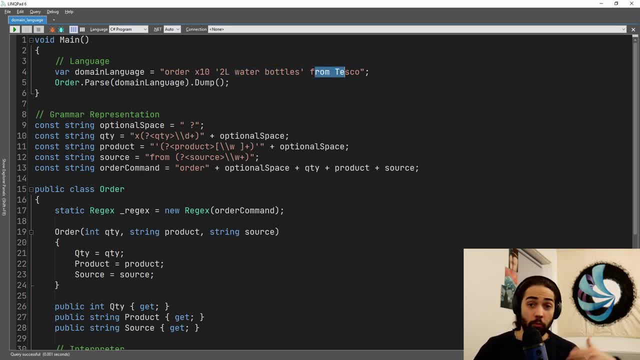 10 eggs, of two liters of waters, of bottles, from whatever shop. the system should be able to create an order and route it to the correct place and then automatically pay for it. So the main distinctions to make here is: we have some kind of language And in our scenario, 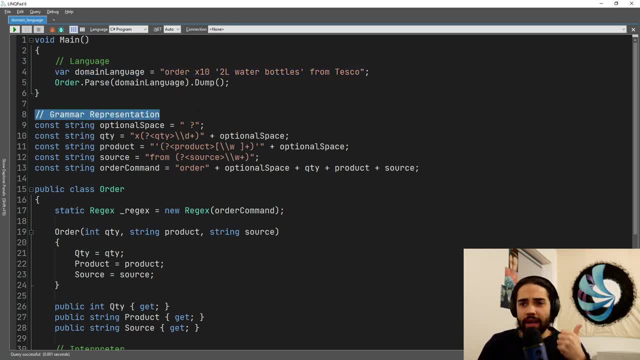 this language could be well understood by anybody. Then we have the grammar representation. Now this is going to look very, very funky if you don't understand regex. and you don't understand regex named capture groups. Otherwise, this should be pretty self-explanatory If you don't know regex. 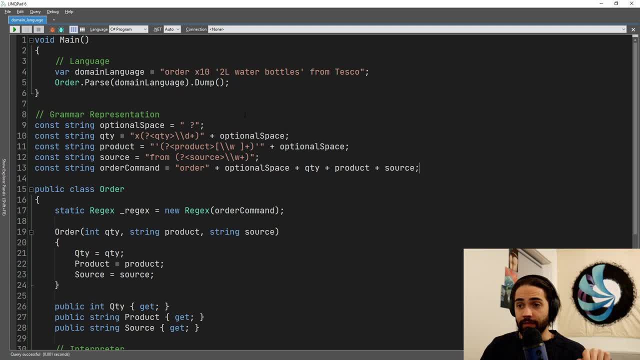 and you want me to make a tutorial on regex, leave a comment. Nevertheless, I've put- hopefully I've put- quite descriptive names Here. we have an optional space, right, So you can put a space or you cannot put a space. It depends on what you want to do. But essentially we have some kind of 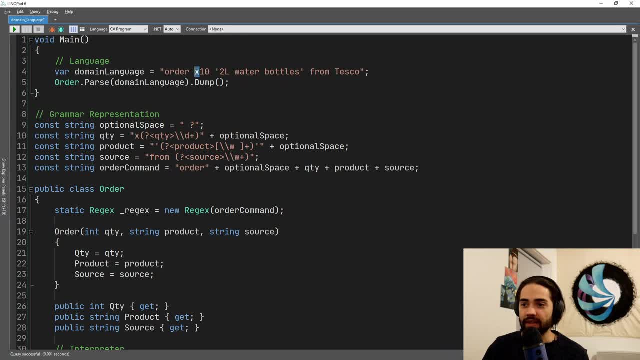 quantity. So X stands for this, X backslash, backslash D plus multiple digits. that will stand for this number And that is what I'm capturing in this group. So later on, when I want to extract the value from the string, that's what I want to extract. I want to extract this. 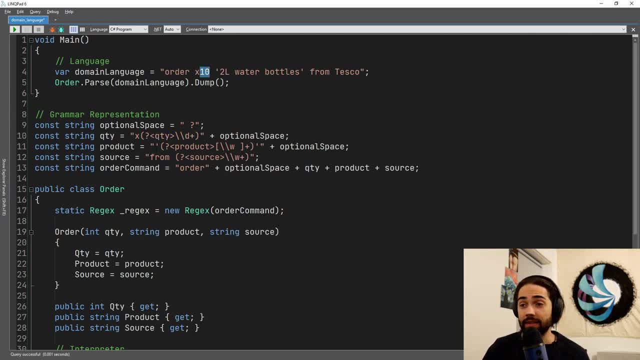 quantity, And when I say give me the quantity, it will give me this number. Next thing is the product instruction, where in my single quotes I will have again a product group And when I query for a product it will give me whatever is contained in these quotes here. Finally, I have 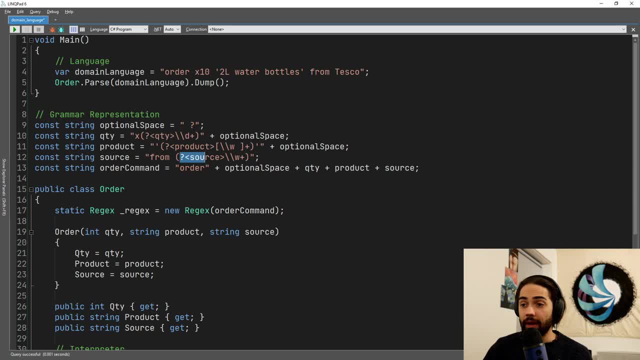 the source. Where do I want to order from? From and then again source. So when I ask for the name of the source, I only have the name of the product. So if I want to order from the product, I have the name of the product And then finally I have the word, the number and the space. So 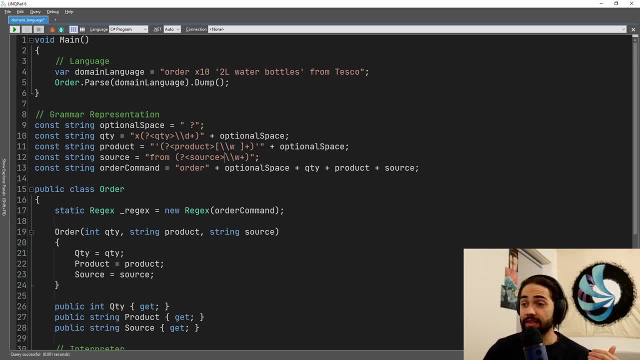 you can see, I included this space, So one or more of these, here, for the name of the source. I only have words, So if this would have had a space, it would break, But nevertheless, for this example, this will do. And then, finally, I comprise the whole order out of these grammar pieces, The point. 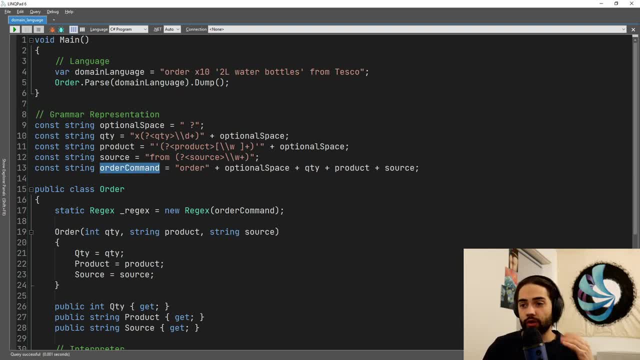 is that we can have multiple commands, not only an order command where I have order optional space, quantity, product source. So we order a quantity of some product from somewhere, We can sell a product from some kind of source to some kind of customer right. We can comprise infinite. 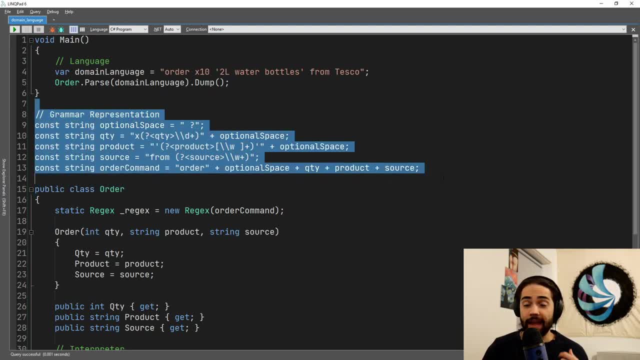 number of grammar representations. That just means sentences that we can interpret At the moment, if we say sell 10 to leader, what Sell 10 to leader bottles from Tesco? and we don't have a command for this, we wouldn't know. 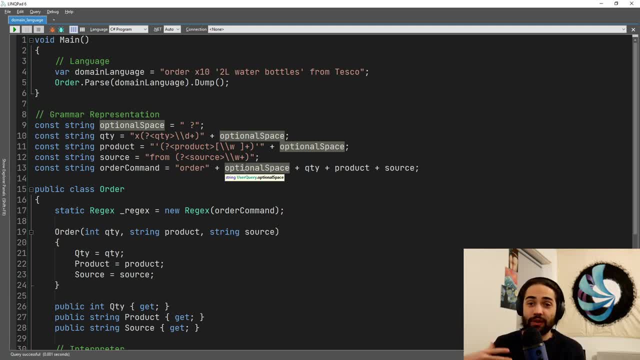 how to interpret it. So this is where our design pattern we're trying to apply, Not necessarily that we're applying it wrong. It just doesn't know how to parse it. It doesn't know how to understand it. It's as if you would have invalid syntax in your C-sharp code. We cannot compile it. 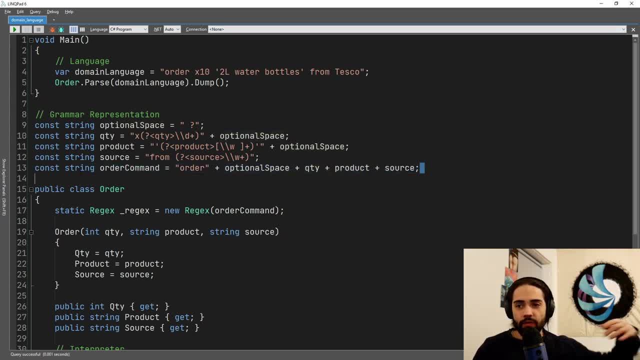 Okay, But hopefully you get the picture. We can create infinite numbers of instructions that we can parse. So if I talk to my Alexa or whatever, and she knows what I'm doing, I can compile it. She understands that she can create this string. She should be able to file the order and pay for. 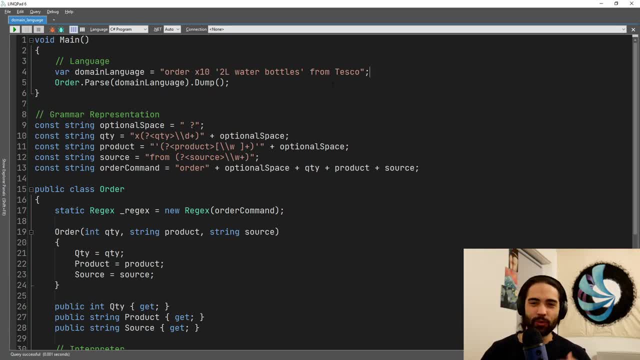 it automatically. Okay, So I don't have to go online, fill out some form, wait for my internet to load, whatever Crazy process, right? Anyway, we have the domain language, So we have the language, the language that we speak, and then we have the grammar representation. So this is how. 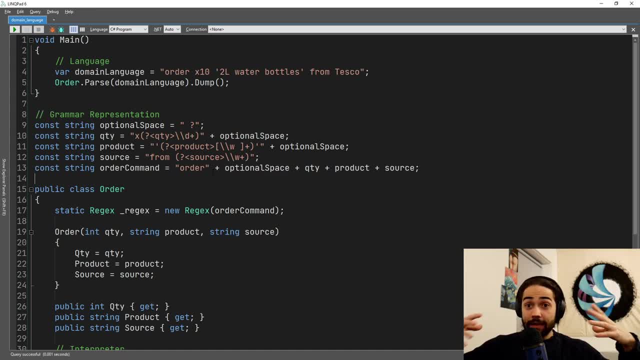 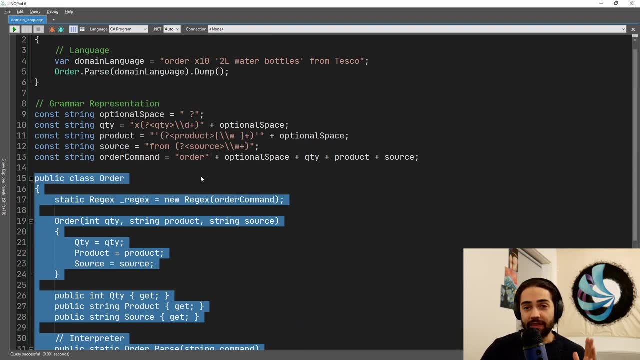 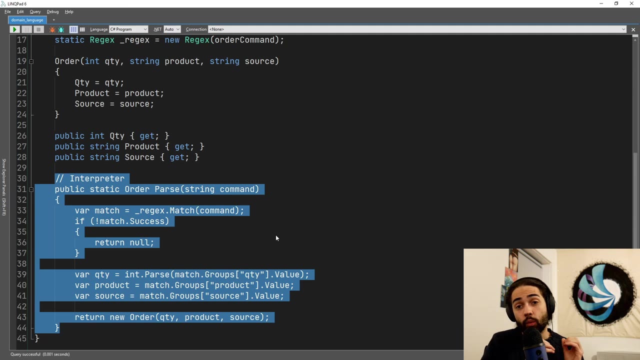 we can represent all possible sentences that we can expect, Okay, And then I have a order. At the moment, this is a very, very simple thing For the example, and the interpreter lives in this function In a real world scenario. 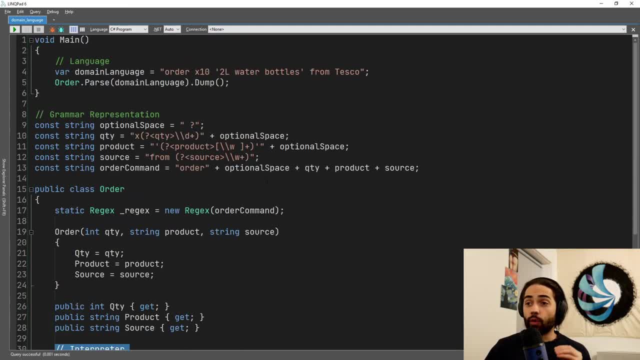 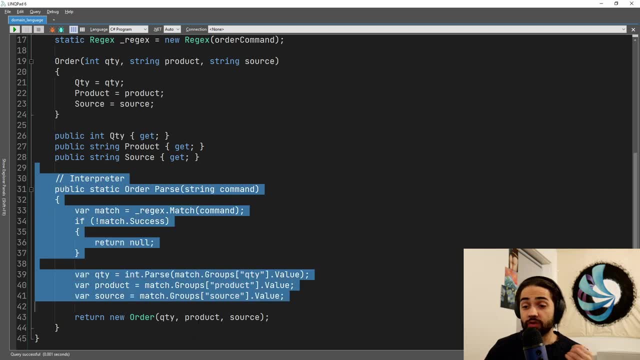 what you're going to end up with is a dedicated object for parsing the language using the grammar into some kind of code. Right now I'm opting in just for a function because I want my example to be as simple as possible And it only does sort of string to object mapping. It doesn't do any. 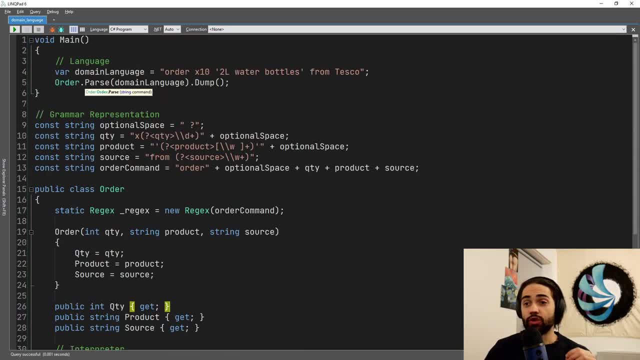 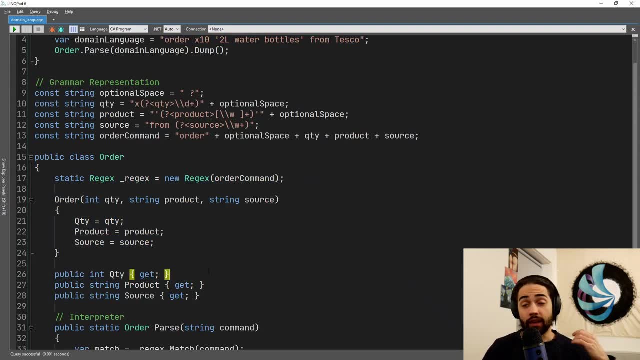 functionality. Hopefully you have enough imagination to understand that it's a function that you can use, So let's go ahead and do that. This language can not only be mapped to a data representation object, It can also be mapped to functionality. same way, your code, your C-sharp code, gets mapped to machine language and gets: 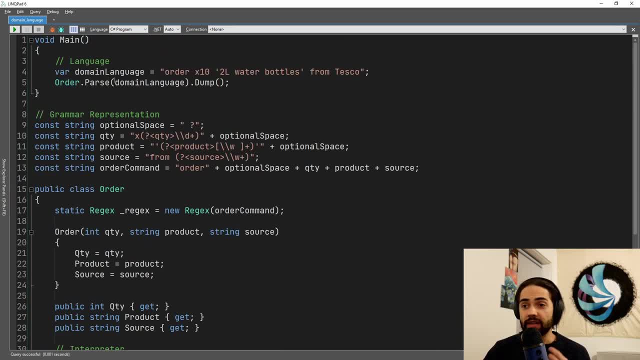 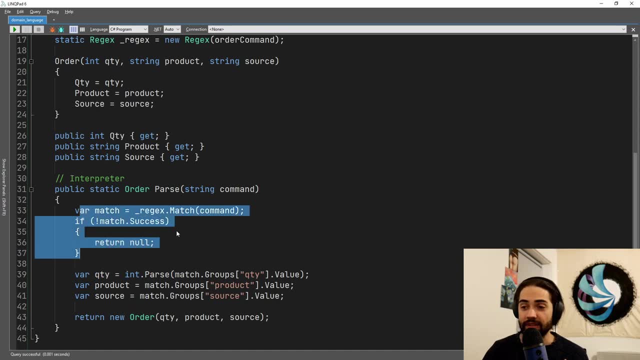 executed on a computer. Here, all we're doing is we're taking the order, We're parsing the domain language and the way that I explained how I take out these parameters. That's what happens here. So I take the regex where I said that the order command is the regex that I want to run. I run. it again, And I'm going to run it again, And I'm going to run it again, And I'm going to run it again, I'm going to run it again, And I'm going to run it again, And I'm going to run it again, And. 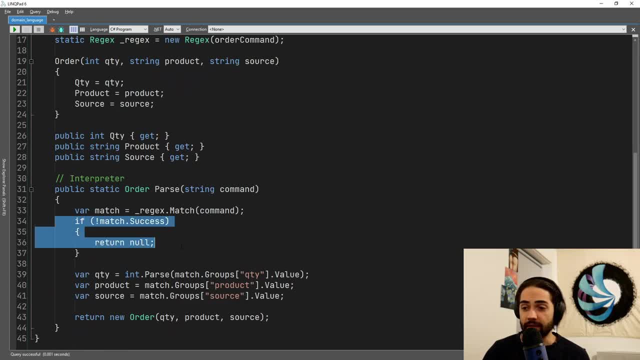 again, And I'm going to run it again, And I'm going to run it again, And I run it again, And I'm going to run it again, And I'm going to run it again. So you get to run the computer and then I run a script where we have to değilog. 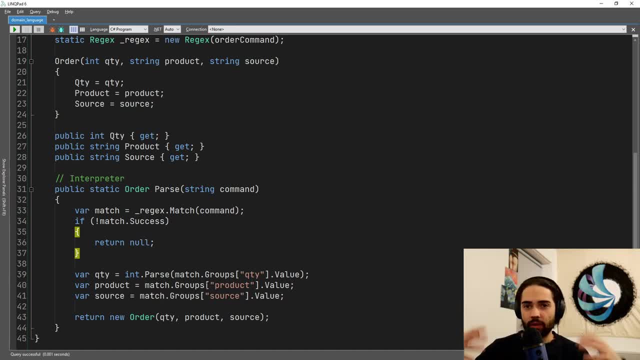 and an overflow ofix support And we can send off this data to Windows. and I'm going to run this data And it will send it back to Windows. You seeds a Logistics for updates and then you're done. So the zadliger side of it is that we can run in 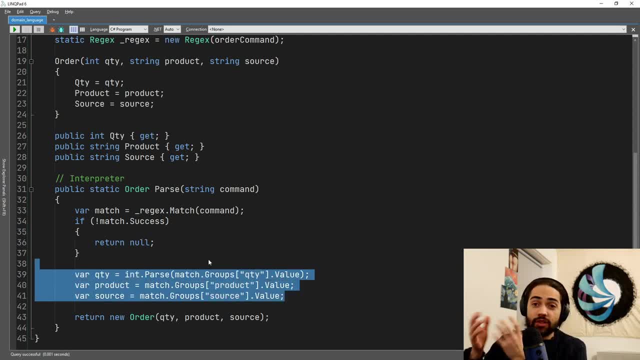 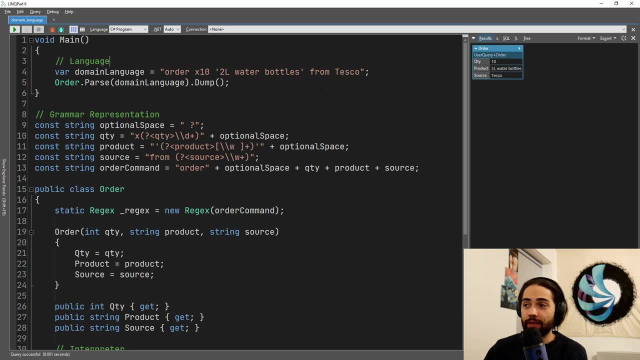 the next stage of üzeri of the command. and then you say you want to run your dos module design here. We hope to just give this a 9-. 왜� it never turns to blue? And now we've got our different the end. If we're on this, we go ahead and get our order with quantity of 10,. product: 10 liter. 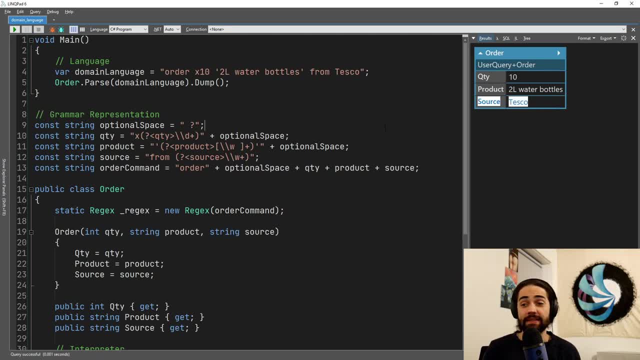 water bottles and source from Tesco. Now this specific example is again on the business side and doesn't contain any functionality. We're literally taking a string and representing it as a C sharp object, right, With just some state in it. More real world examples of interpreters. 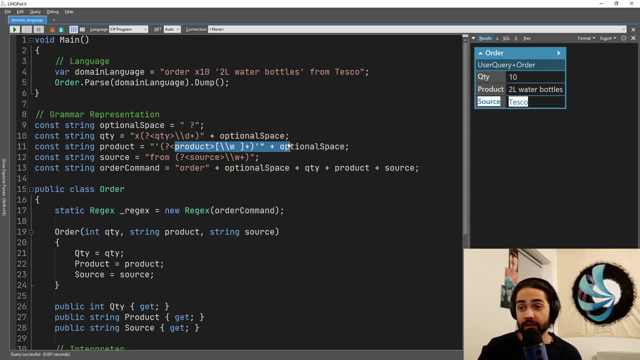 are things like regex, for example. So I've written some. you know crazy language right here, and regex is so widely used that you will find it implemented in all languages outside of languages. It's literally used everywhere and it's the same notation in every language. So you've learned. 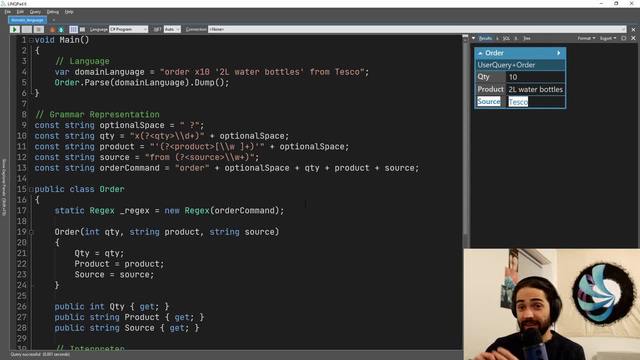 the skill and you're able to use this language everywhere. So it's decoupled from programming. So the language is regex, The grammar are individual signs, groups, characters, Special characters, etc. That's the grammar right, Same as in Russian. we would have different. 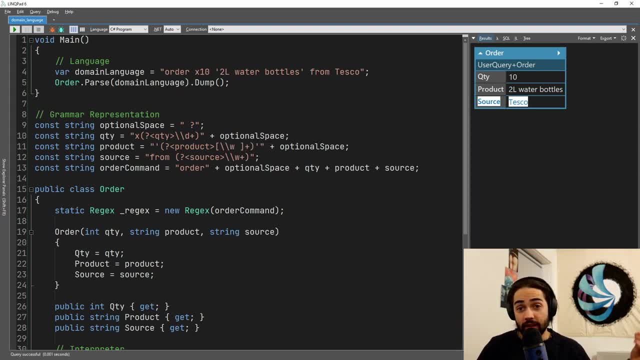 letters. compared to English, It's different grammar Here. in English you wouldn't have backslash, backslash D plus. That doesn't mean too much Once you're speaking. regex, that means multiple, one or more numbers, And the interpreter pattern is just understanding that you have some. 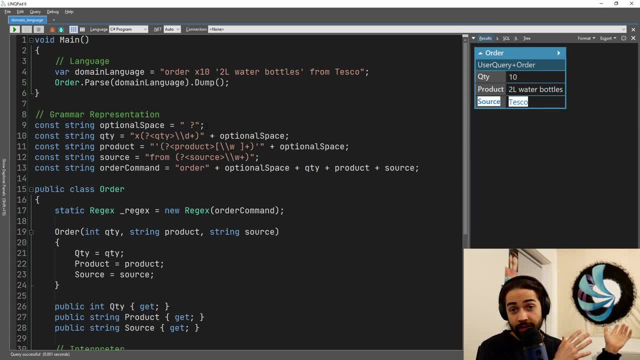 kind of language and you want to map it to some functionality once you parse it And that's it. So not hard to understand, Not hard to recognize. It will be hard to implement and the amount of work will depend on the sophistication of your language. Other good examples of interpreter patterns is essentially 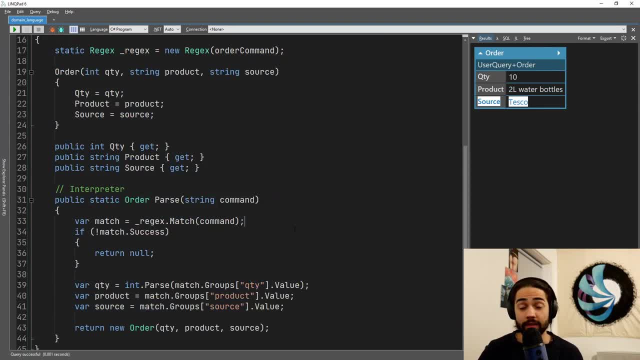 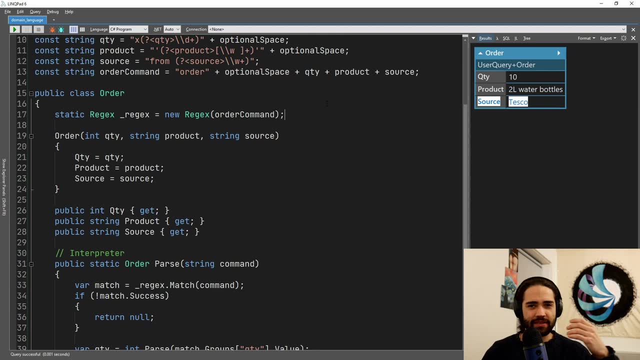 having a language like C-sharp and then the compiler using an interpreter to interpret whatever code you have written here. This will be same for Java, C++, Python, Clojure and a plethora of other programming languages. All compilers have interpreters to understand what they're doing, So it's a good example of how you can use a language like C-sharp.